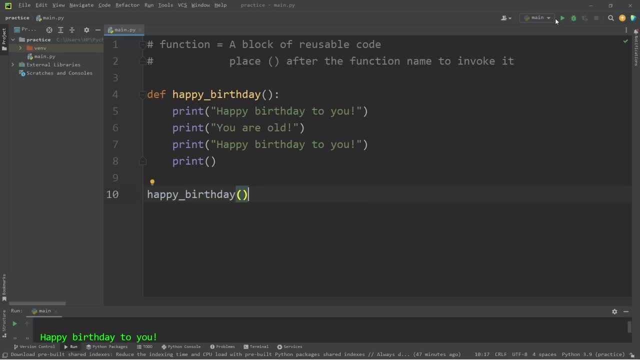 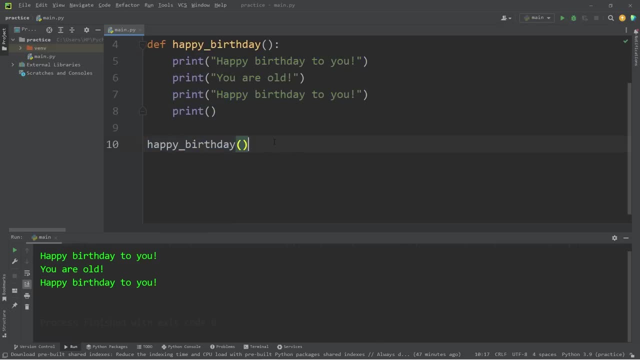 happy birthday, add a set of parentheses and that's it. When you invoke this function, you will execute this code once. If I need to execute this once, I will execute this code twice. code three times. I would just call it two more times. Happy birthday, happy birthday, happy. 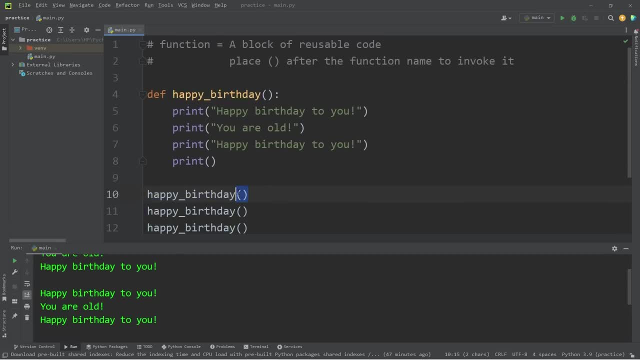 birthday. To invoke a function, you type the function name, then add a set of parentheses. I like to think of the parentheses as a pair of telephones talking to each other. You call a function to invoke it. Hey, happy birthday. function. execute your code. 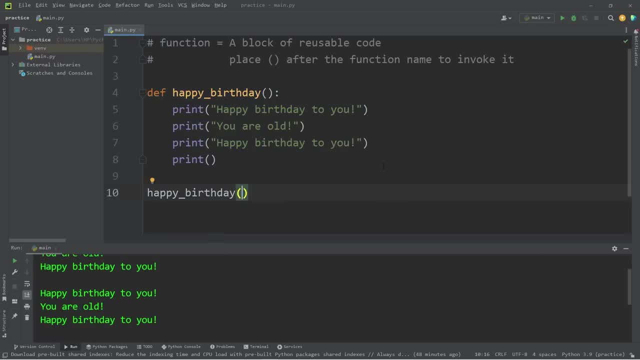 With functions, you are able to send data directly to a function Using what are known as arguments. you can send values or variables directly to a function. Place any data within the set of parentheses. I'll send my function a first name. Any data you send a function are known as arguments. 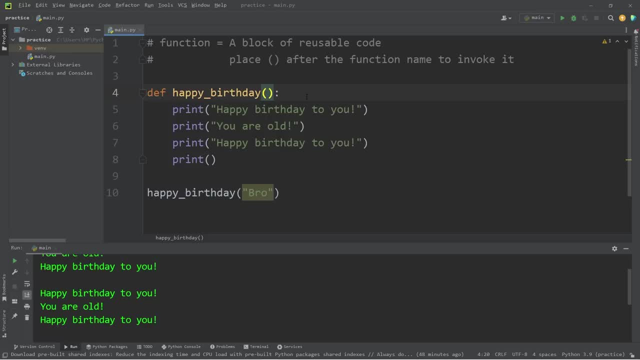 but you need a matching set of parameters that are in order. What exactly is the data we're sending in? Well, it's a name. I will add one parameter to my happy birthday function. I will name this data name. A parameter is kind of like a temporary variable that's used within a function. 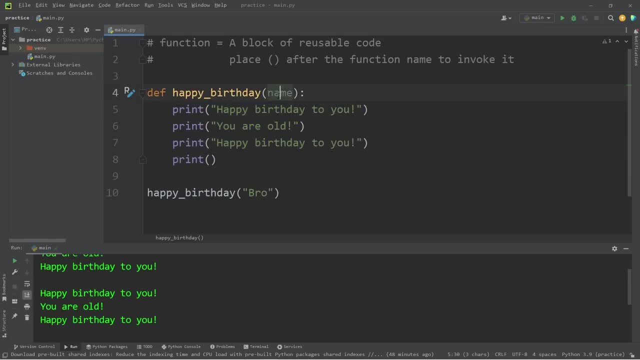 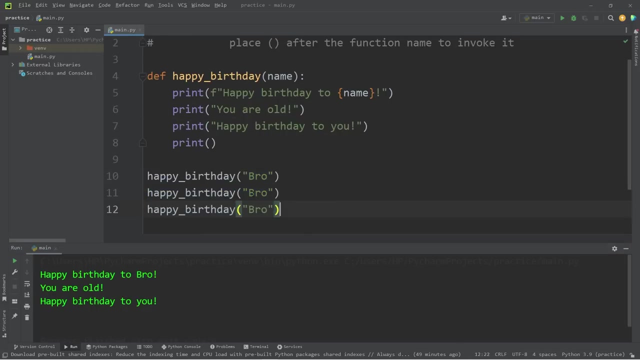 I'm going to replace this instance of you with a name. I will use an F string. replace you with a placeholder. I will add my parameter name. So, happy birthday to bro. We could pass in some other names. What about Steve and Joe? 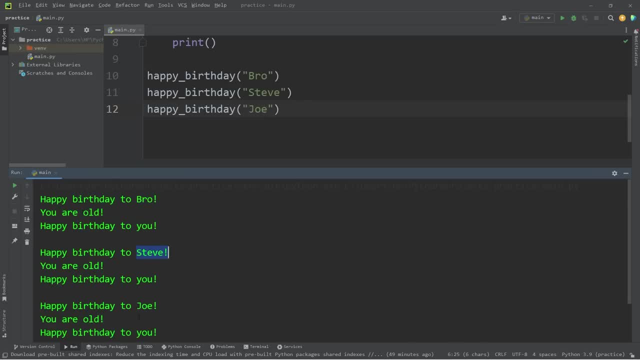 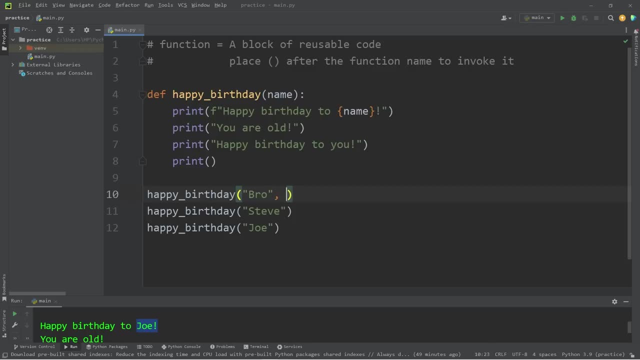 Here we are: Happy birthday to bro, Happy birthday to Steve, Happy birthday to Joe. When you invoke a function, you can send more than one argument. Let's send an age. this time I'll send 20,, 30, and 40. But when I run this we have an error. We're passing in two arguments. 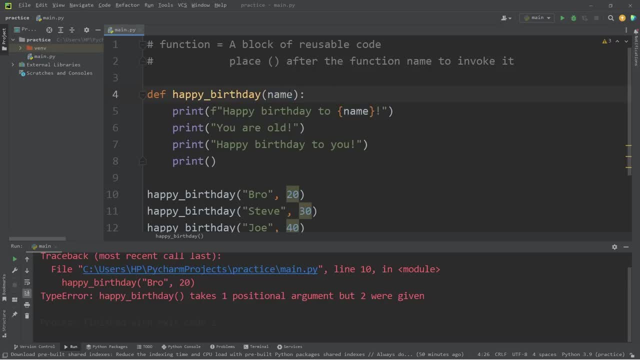 but our function is set up only to take one. I would need a matching number of arguments To invoke this function. we will need two parameters. We have a name and we have an age. Then let's use this: this age You are. let's make this line an f-string age: years old. Let's try that again. 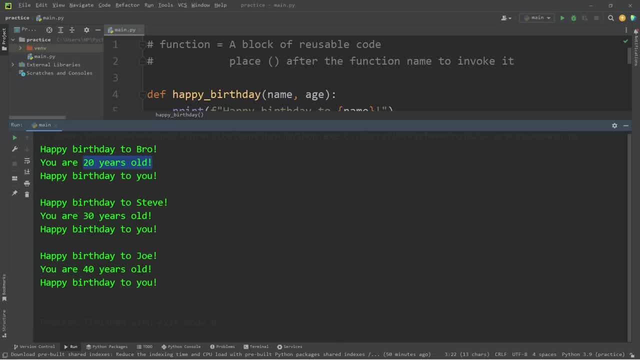 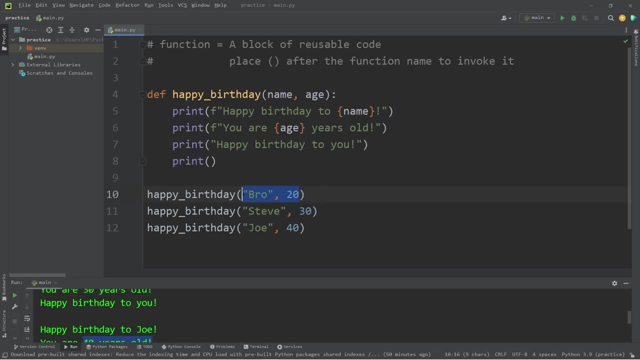 Happy birthday to bro: You are 20 years old. Happy birthday to Steve: You are 30 years old. Happy birthday to Joe: You are 40 years old. When you invoke a function, you can pass in some data- Those are known as arguments- but you'll need a matching set of parameters. The order does matter. 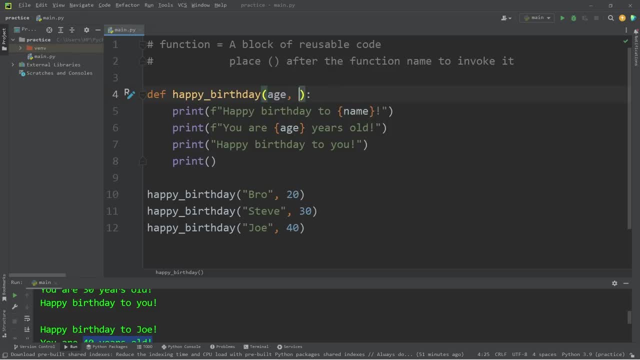 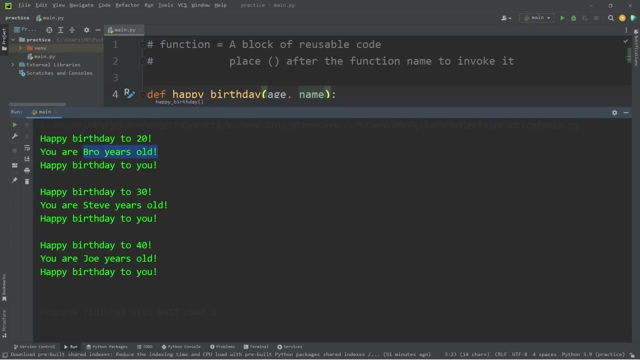 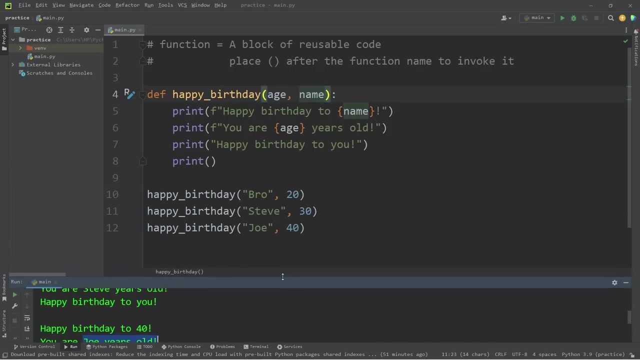 Let's see what happens when I switch these two parameters: Age, then name. Happy birthday to 20.. You are bro years old. Happy birthday to 30.. You are Steve years old. Happy birthday to 40.. You are Joe years old. So the position of the parameters does matter. 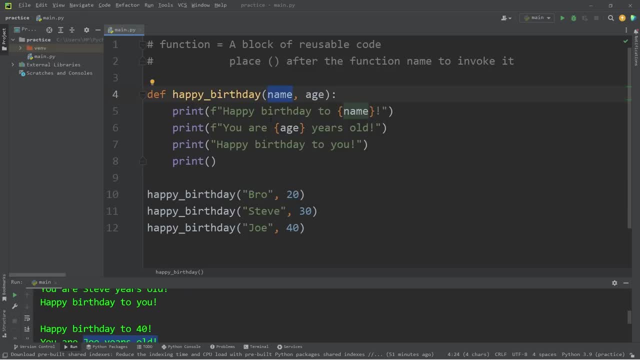 Same thing goes with the arguments. You also could name these parameters something unique, Maybe x and y. Happy birthday to x. You are y, You are 20 years old. That's also valid. Let's try another example. I'm going to create a function. 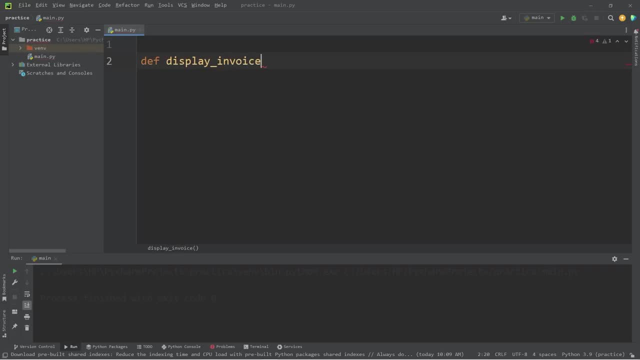 to display an invoice, There will be three parameters: A username, an amount and a due date. Let's print hello. I should make this an f-string Username. We'll use another f-string: Your bill of amount. Let's precede this placeholder with the unit of currency. 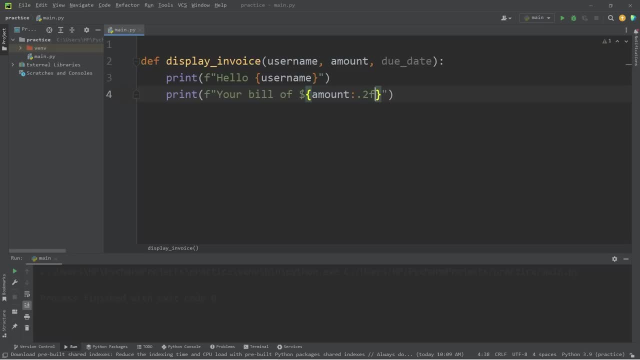 I will also add a format specifier Point to f is due on our due date. Whatever that parameter is To invoke this function, we will type the function's name, Add a set of parentheses, A username, An amount And a due date. 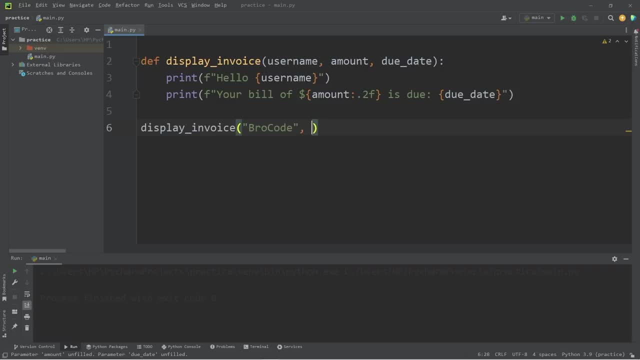 Let's make up some username, An amount, I guess $42.50.. I'm just making up a number here, Then a due date: The first of January, I guess. Here is my invoice. Hello, brocode, your bill of $42.50 is due on January 1st. 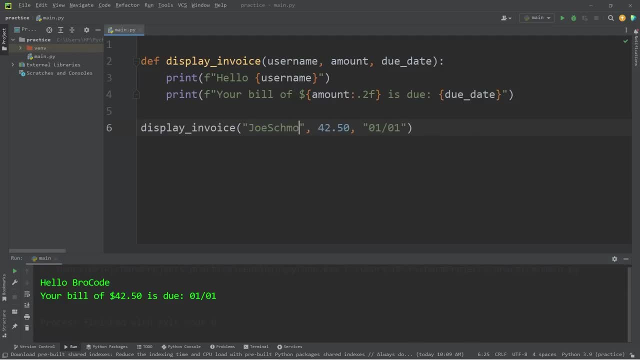 Let's change these arguments. Joe Schmoe is the username. He owes $100.01.. Due on the 1st of February Or January 2nd, depending on how you read dates in your region. Hello Joe Schmoe, your bill of $100.01 is due on 1-2.. 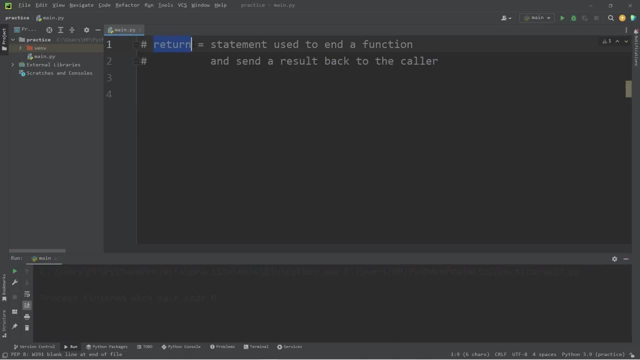 That's another example. Now we need to explain the return statement. Return is a statement that is used to end a function and send a result back to the caller. Here's an example: We have a variable, z. z will equal. We'll invoke a function to add two numbers together. 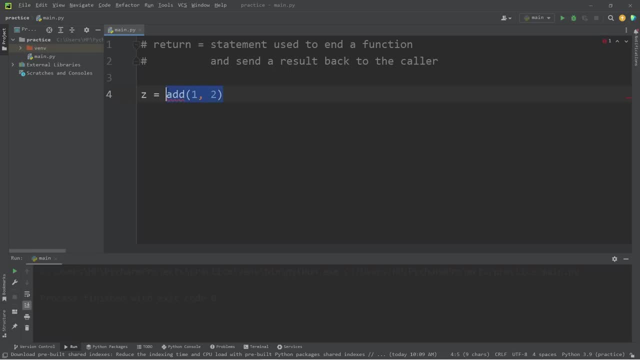 Such as the numbers 1 and 2.. When we invoke a function, we can send some data back. After adding 1 and 2, we will send the result, Which would be 3. Then this value can be assigned to a variable. 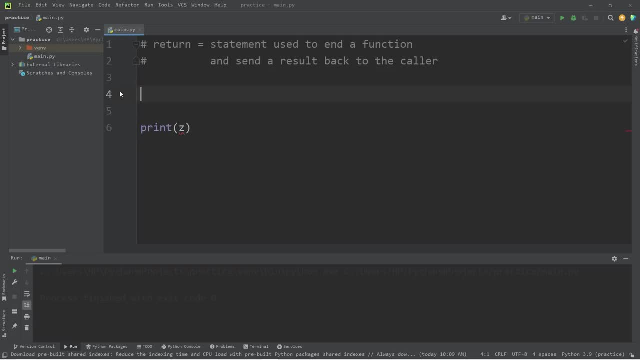 Then we can print whatever z is. So let's create some functions. Let's create a function to add two numbers together. The parameters will be x and y. Let's say: z equals x plus y, Then we will return our value z. 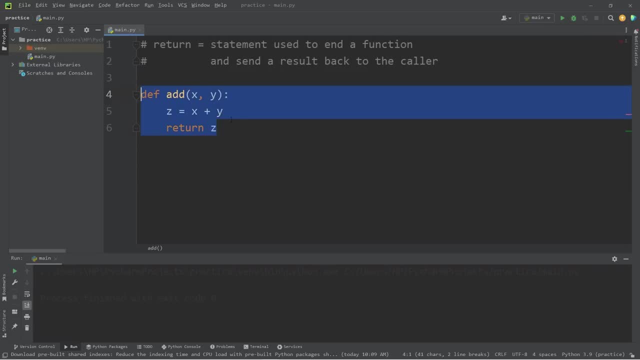 So I'm not going to print z directly right now. Let's subtract x and y. Subtract z equals x minus y. Return z. Multiply x times y, Then divide x divided by y: Return z. Let's invoke our add function. 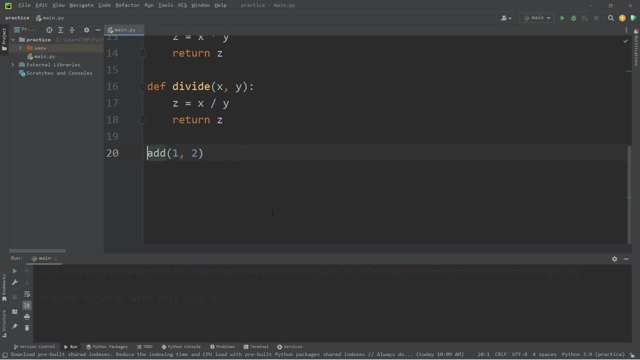 Pass in two numbers: 1 and 2.. Then I'm going to print the result After adding these two numbers together. The result is 3.. What about subtract? Subtract 1 and 2. The result is negative: 1.. 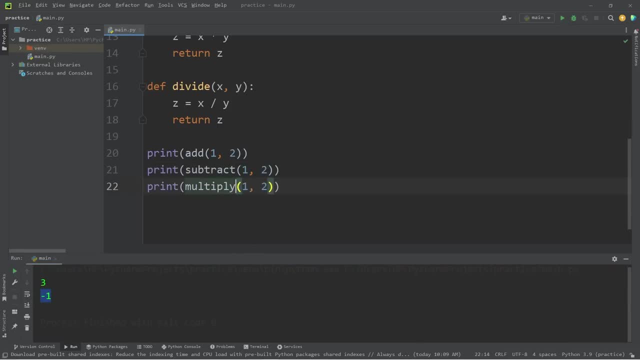 Multiply, The result is 2.. Then divide 1. divided by 2 is 0.5.. After we resolve this function, A value is returned. Just imagine that after we finish this function, This function becomes whatever is returned, 3.. 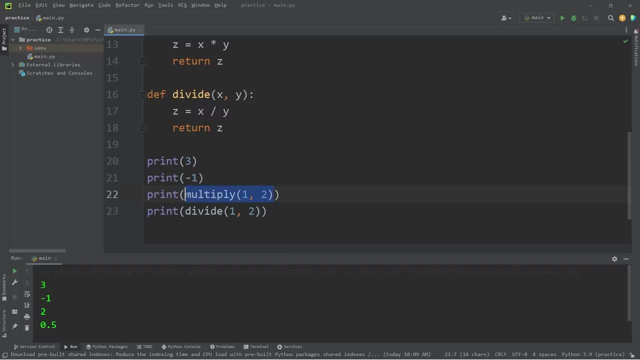 This function becomes negative. 1. This function becomes 2.. This function becomes 0.5.. Let's write something a little more complex. We will create a function to create a full name: CreateName. We'll need two parameters for a first name and a last name.